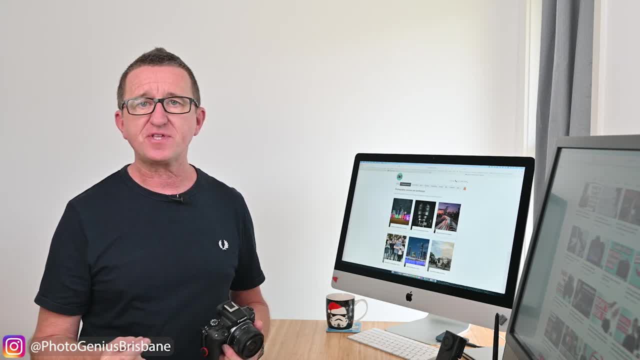 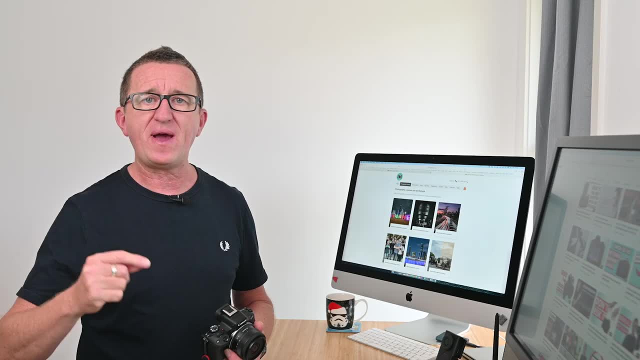 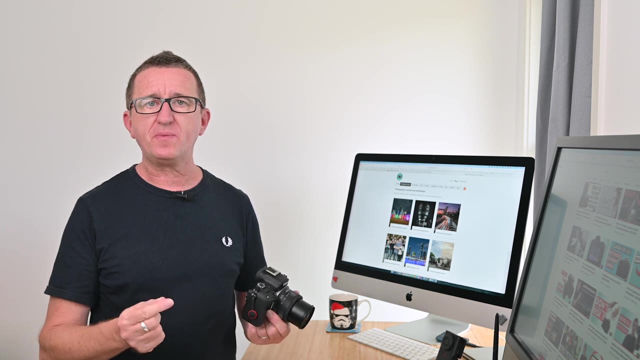 if you are a beginner, then the program mode, I think, is a great option to get you started. So select P on the mode dial and I'll talk a little bit more about what the program mode can do later in the video. Now, with the camera turned on, what's displayed on the screen will depend on. 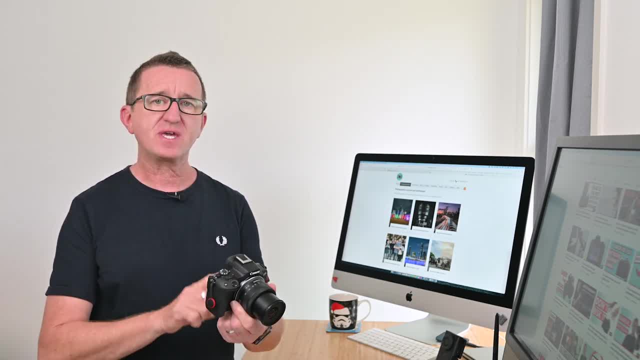 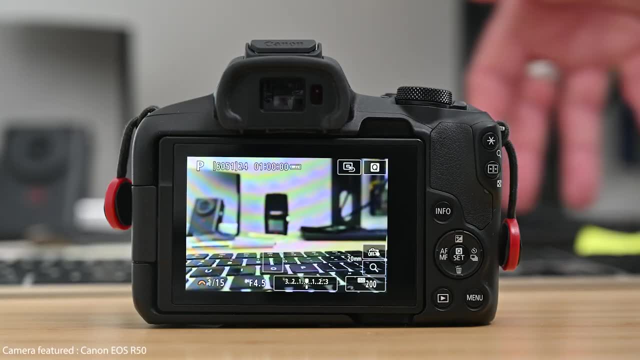 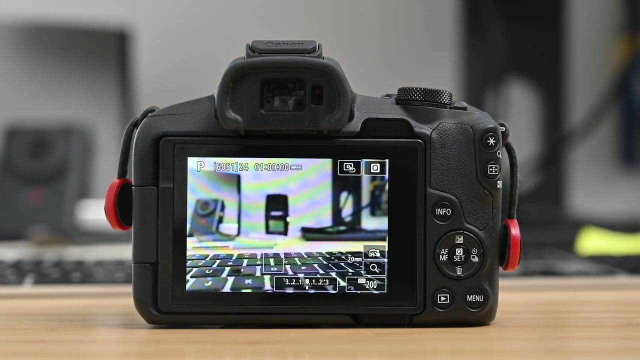 what camera mode you're using, but typically what I see on the LCD screen is what the camera sees via the lens, and we call this live view. So if I wave my hand in front of the camera, you can of course see my hand on the screen in real time. hence the term live view. Now to save battery. 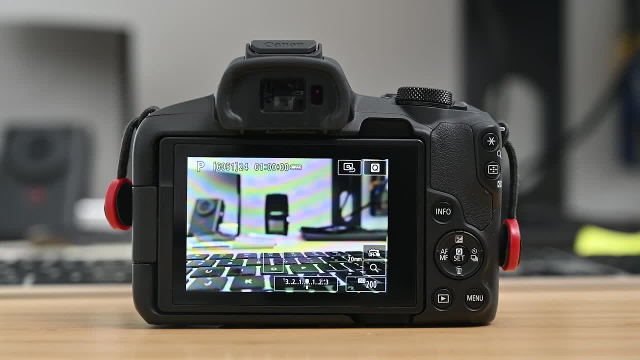 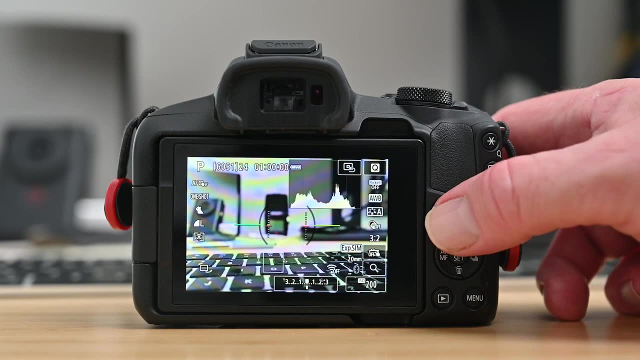 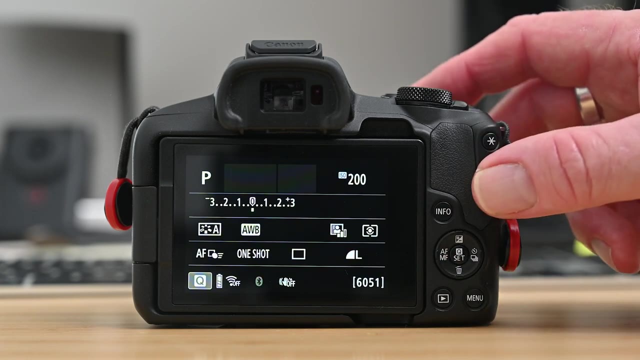 my tip is to change what is displayed on the screen, And you can do this by pressing the info or display button. Each press will change what information is displayed on the screen, and eventually you should see something like this Now, whilst this screen can look a bit intimidating at first, once you start getting familiar with the 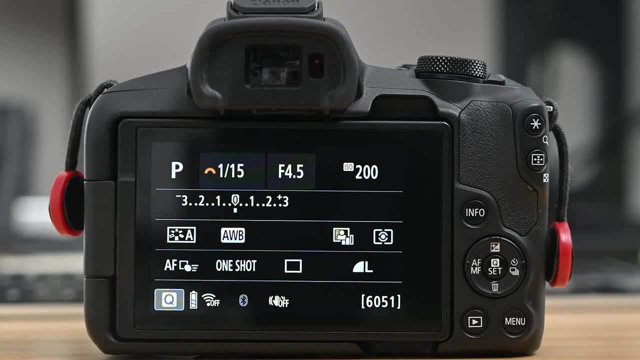 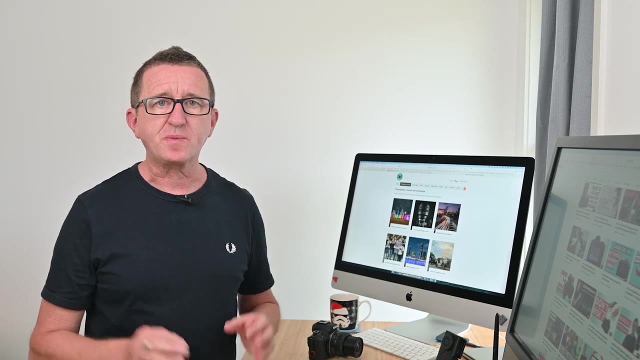 camera. you will find that this screen is very useful, as it clearly displays the current camera settings, such as shutter speed, aperture and ISO Plus. we are extending the battery life Now. we don't need to worry too much about these features at this early stage, but it is worth. 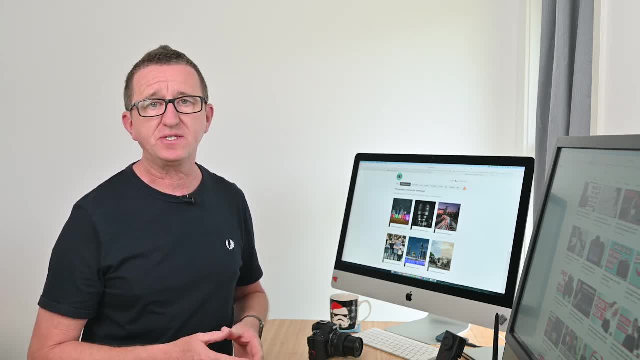 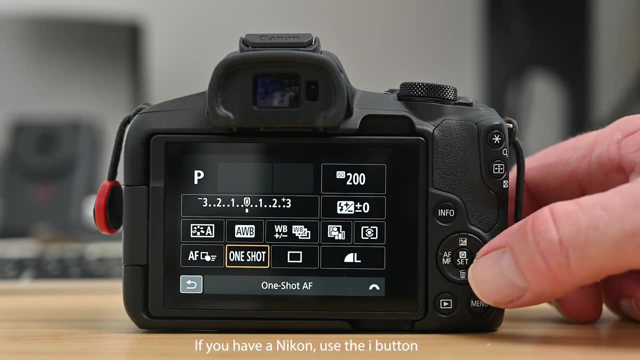 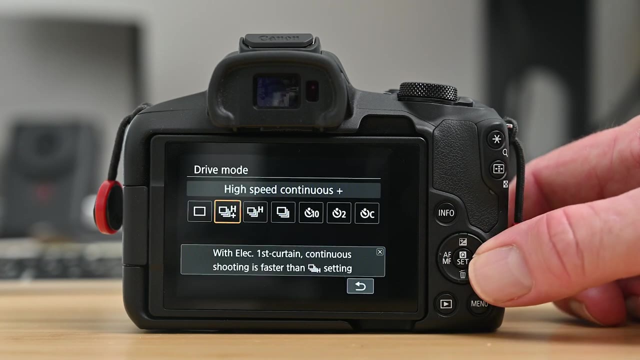 knowing that if you should wish to change any of these settings, you can do very easily using the Q button. So, for example, push the Q button and use the surrounding four buttons to move around the screen. Here, for example, is the drive mode. You can use this to set the camera to take. 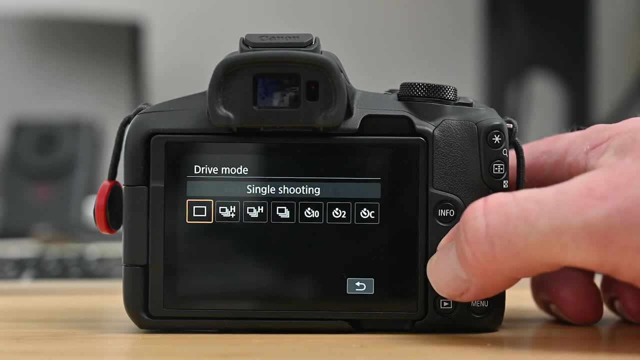 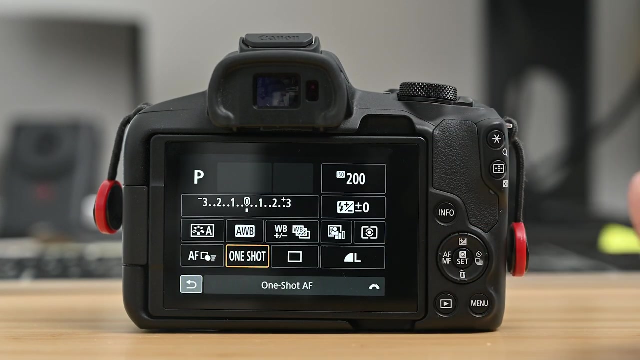 multiple photos or set up a self timer. Next to that is the focus mode. One shot is the default option. Servo is great for moving subjects. Now some cameras, like this one, may also have a touch screen. You can then select Q via the screen and select and change any of the camera modes, all by using the touch screen. 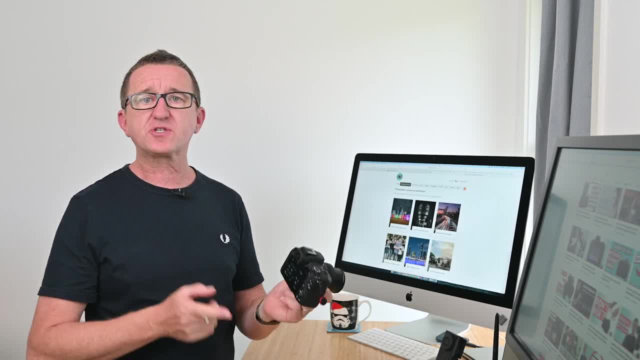 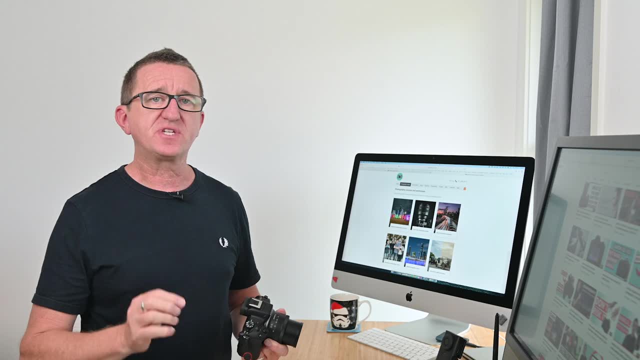 Now, if you put your camera up to your eye and use the viewfinder, the screen should turn off automatically and you will now see the live view actually through the viewfinder. Now note: if the display seems a little bit fuzzy and out of focus, try turning the dial on the side of the viewfinder. 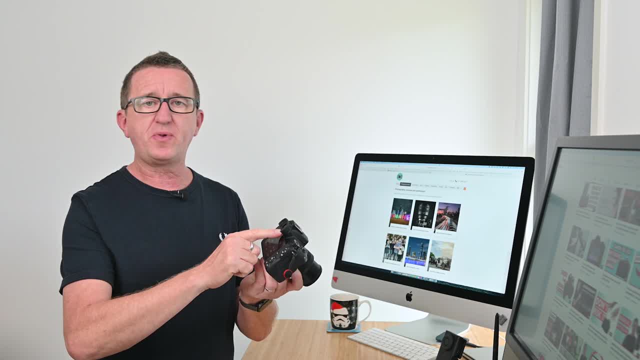 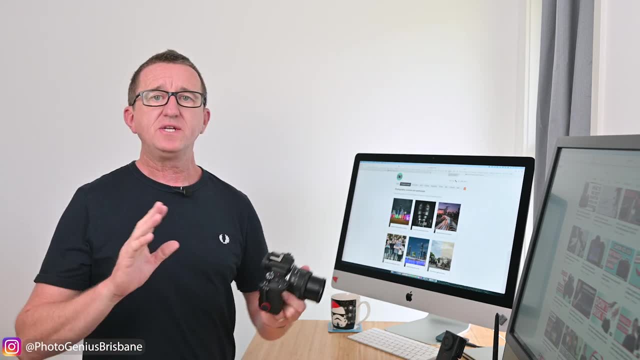 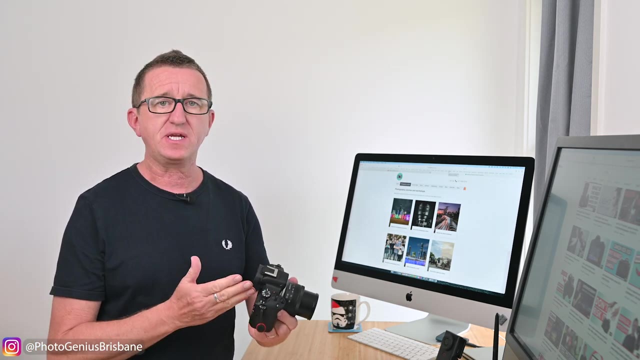 or in the case of this R50, there's a little slider along the bottom and all you need to do is adjust it to suit your vision. Now here's a great tip. if you are using a mirrorless camera, Did you know that you can play back and view your photos or videos through the viewfinder as well as the screen? 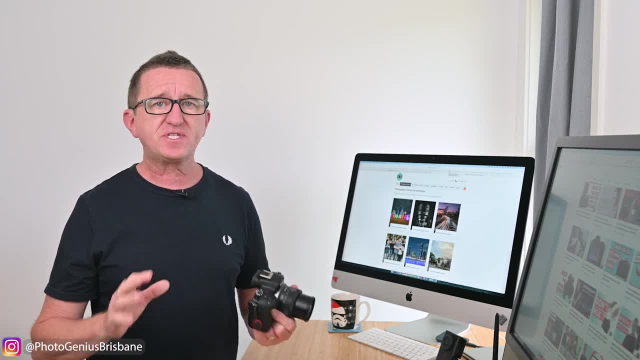 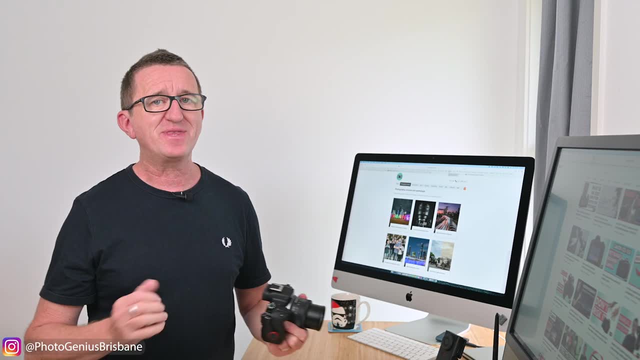 Now, this is a feature that I personally use all the time, particularly if I'm outdoors and it's hard to see the screen Because of reflections. Now, if you're enjoying this video and these tips, can I please ask you a very quick favor? Please consider hitting the like button. you'll find it somewhere down here. 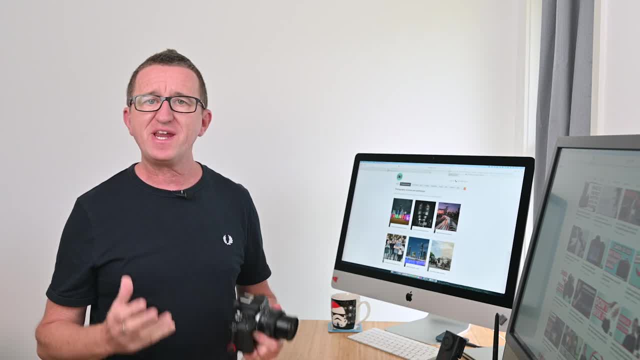 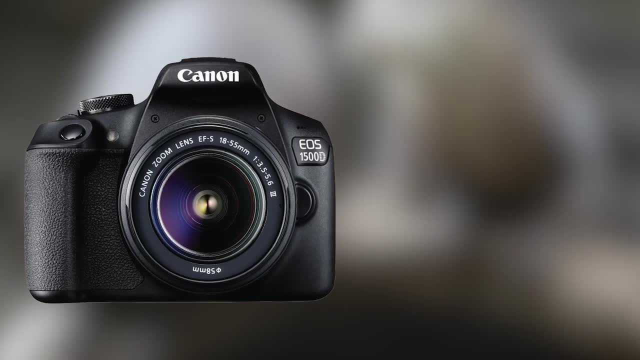 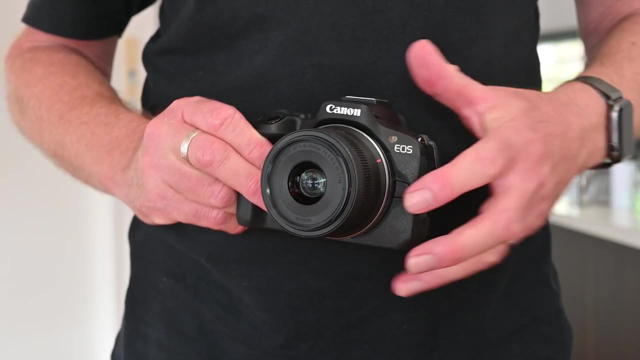 Giving this video a thumbs up costs you nothing, but really helps these videos reach more people. Thanks a lot. Okay, now let's talk about lenses. DSLR or mirrorless cameras like the R50 have removable lenses. The lens can be easily removed by holding down the release button. 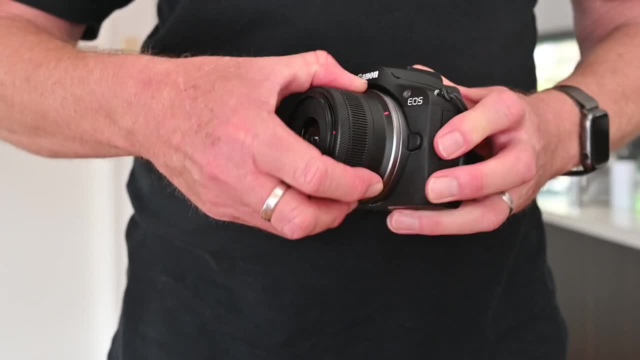 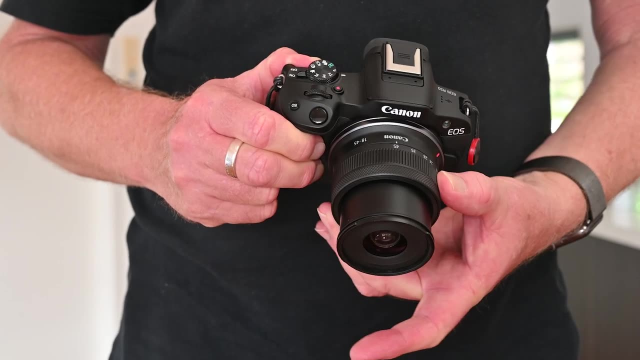 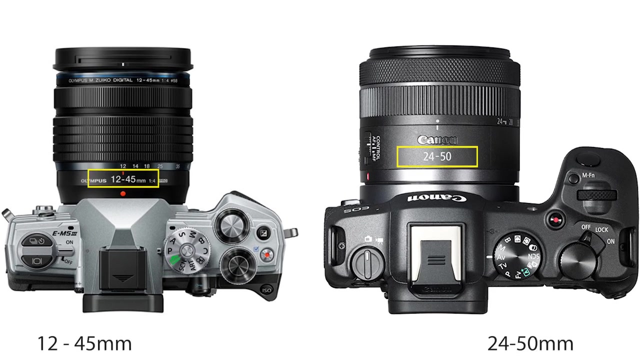 and turning the lens. When reattaching the lens line up the color markers. Now some of the newer lenses have to be unlocked and extended before use and it's likely you will see a message on the screen to prompt you. The numbers on the top indicate the focal length of the lens, also known. 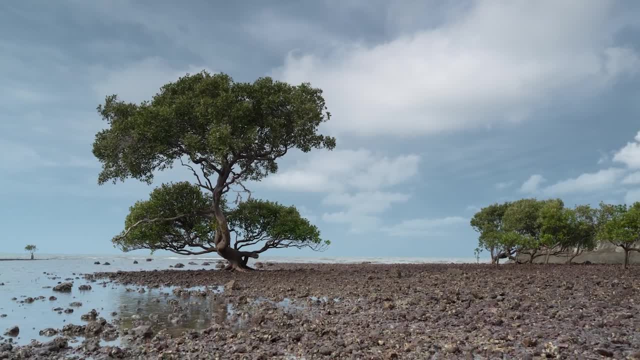 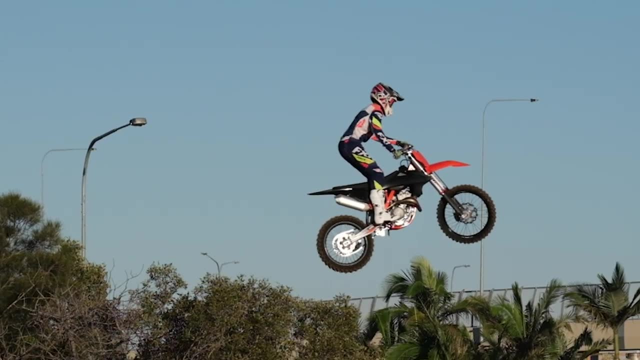 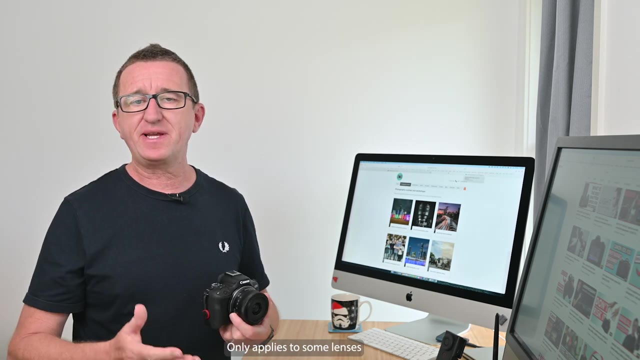 as the zoom range. The lower the number, the wider the view. Turning the zoom ring on the lens increases the focal length, which is also known as zooming in. The subject will now be visible Now, when you're done, rotating the lens back to the lock position of course makes the lens more. 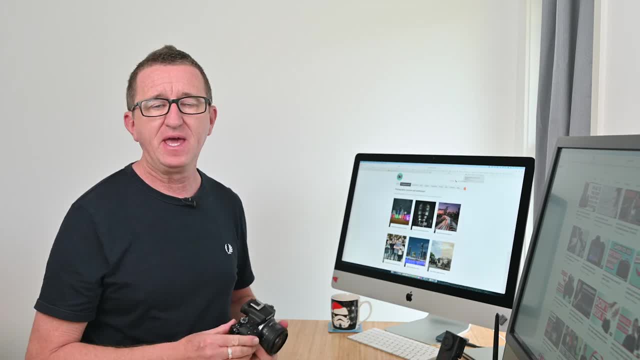 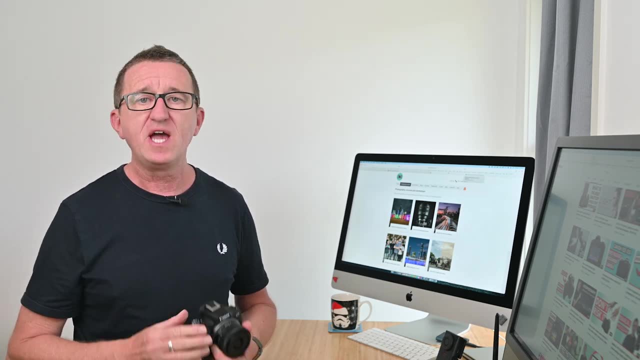 compact, so it takes up less space in your camera bag. Okay, another tip: if you do have another lens, when changing lenses, always try to swap them as quickly as possible to avoid any dust settling on the sensor inside the camera, Because this can cause dust spots to appear in your images. 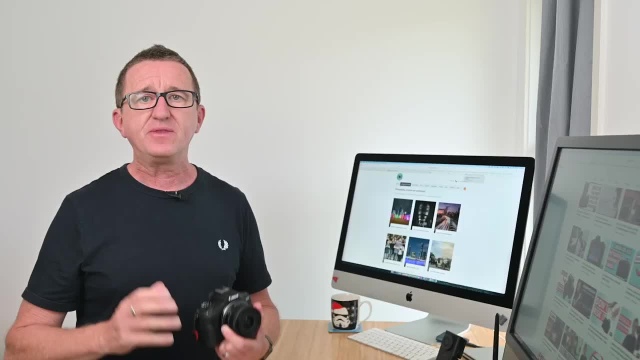 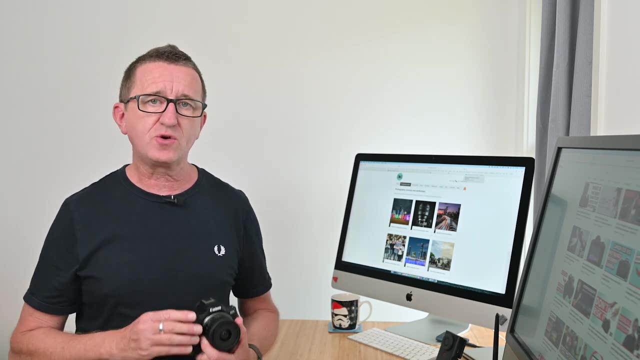 Never touch the sensor. if it looks like it needs a clean, then you can by sensor cleaning kits, but there are also plenty of companies who will do this for you. Contact your local camera store for more details. Now, another tip is if you do have a second lens. 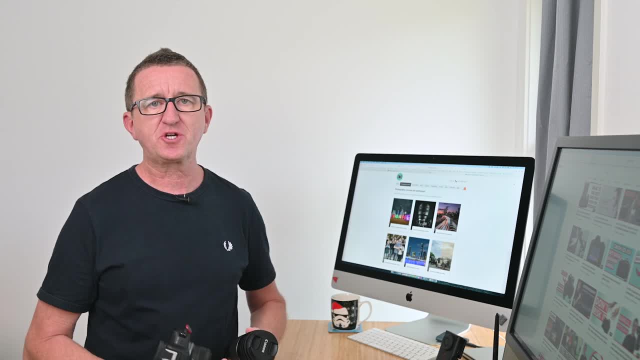 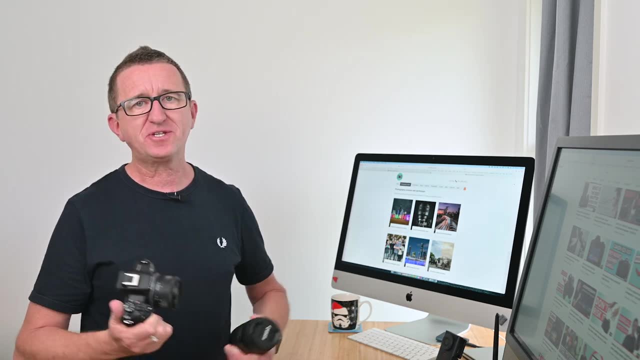 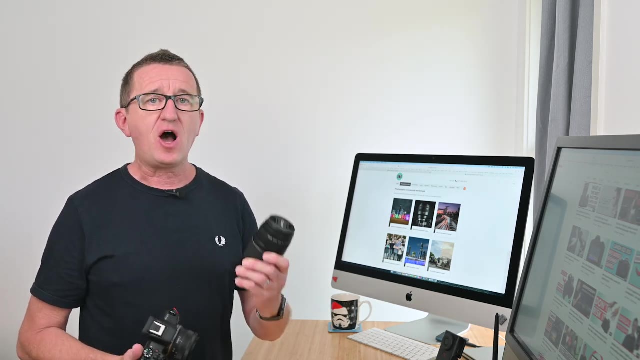 make sure you use it. I meet so many people on my workshops who have a twin lens kit but only use the smaller lens because it's lighter and more compact, which I understand. Different lenses will give you different results. Longer lenses, also known as telephoto lenses, are 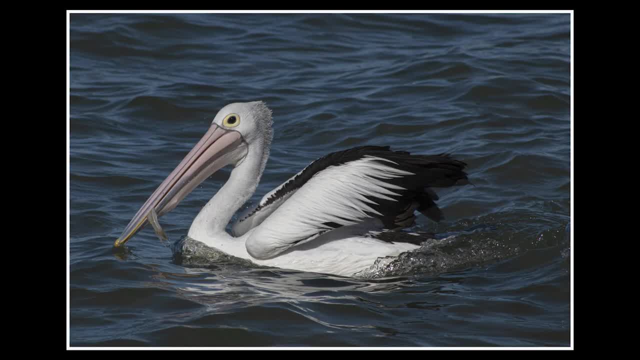 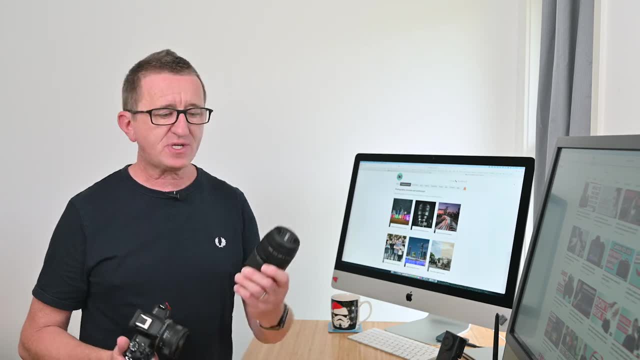 photos of subjects that are further away, but they can also make great portrait lenses too, as they will give you some background blur and compress perspective. So give it a try Now. at the very beginning of this video, you may recall, I suggested selecting program mode, that's 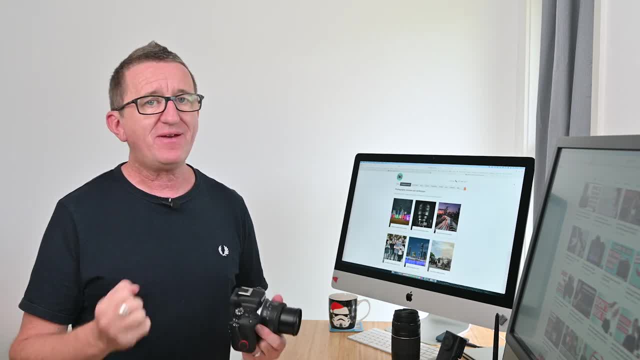 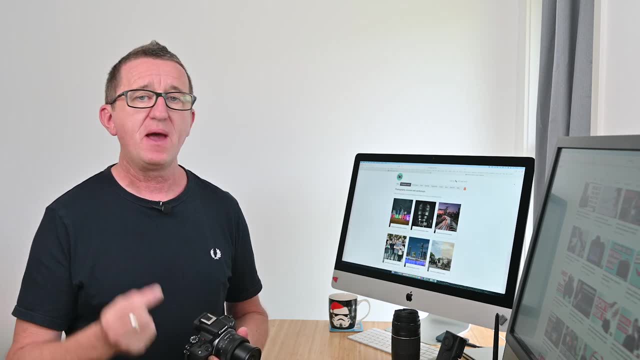 P on the dial as an alternative to auto. Now let's talk about why. So the great thing about the program mode is that the camera will do most of the work for you, but unlike auto, where your options are very small, You can also use the auto mode to take photos of subjects that are further away. 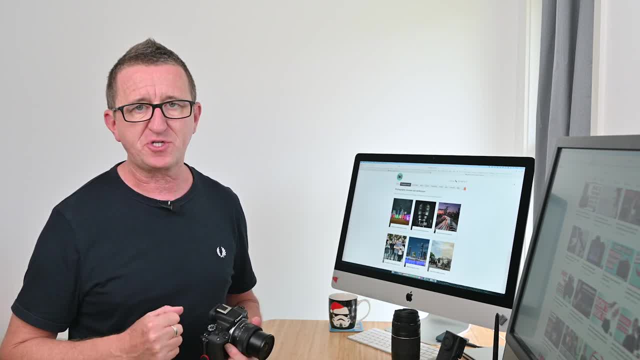 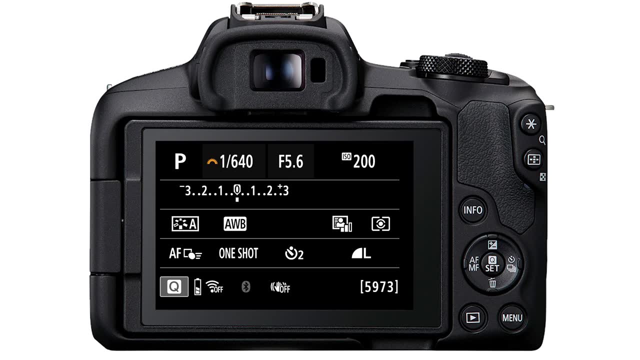 Now let's talk about why. So the great thing about the program mode is that the camera will do most of very limited. in the program mode you will be able to adjust more of the camera's key features. So, for example, with the Canon R50, turning the dial on the top of the camera will adjust the shutter. 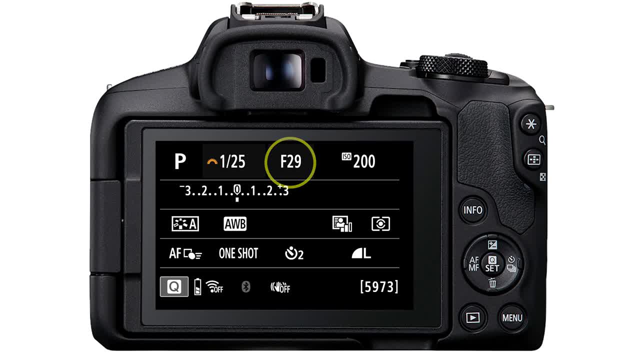 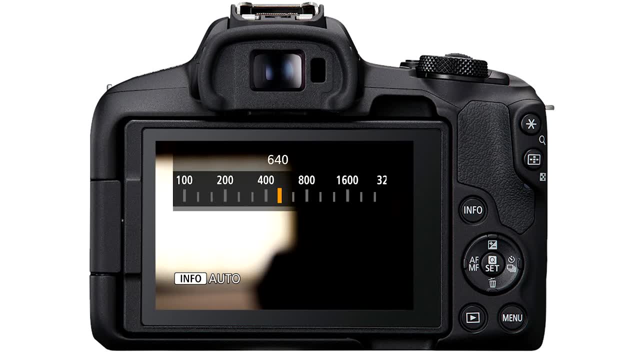 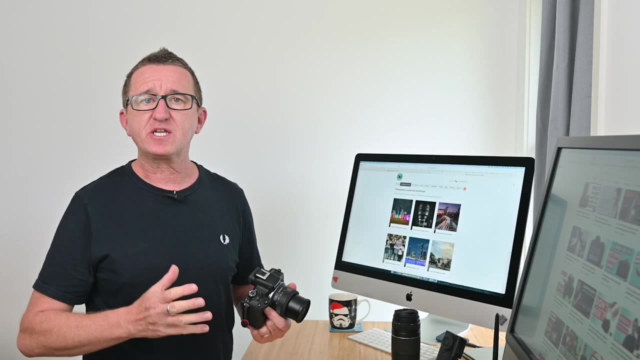 speed with the camera. looking after the aperture Plus, you also have the option to adjust the camera's ISO. This can be used to affect how bright or dark your images are. You cannot do this in auto Now. different shutter speeds will affect movement in different ways, So I think 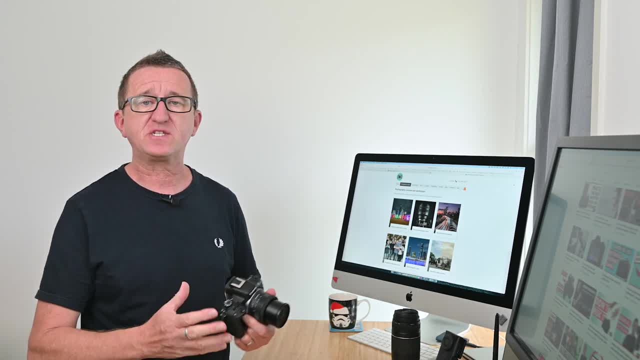 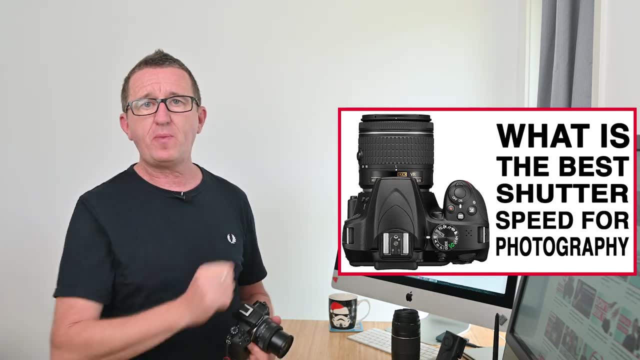 it's best to have a play around with this and get a feel for what works best for you and your subject. Now, if you want to find out more about shutter speed, I suggest watching this video. next, I'll pop a link somewhere up here and also at the end of the video. Now another reason for shooting in the 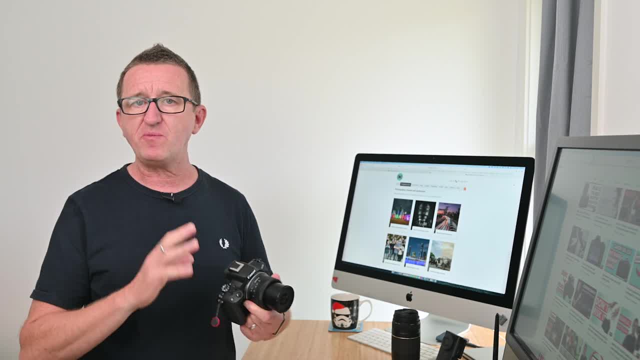 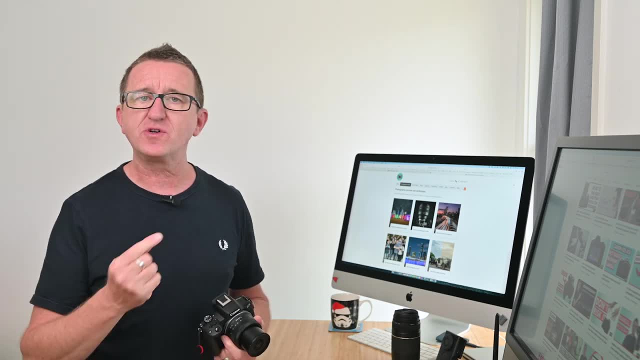 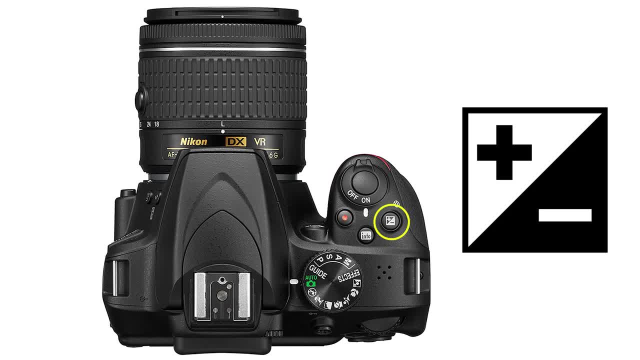 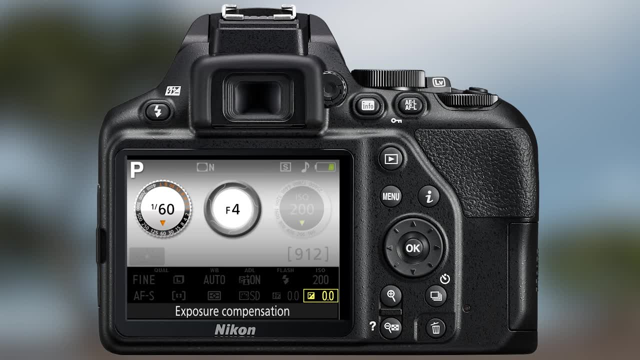 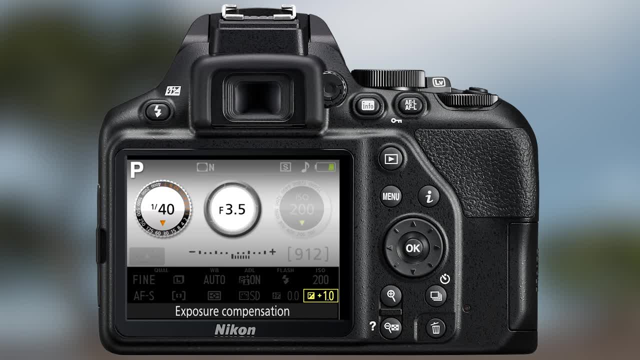 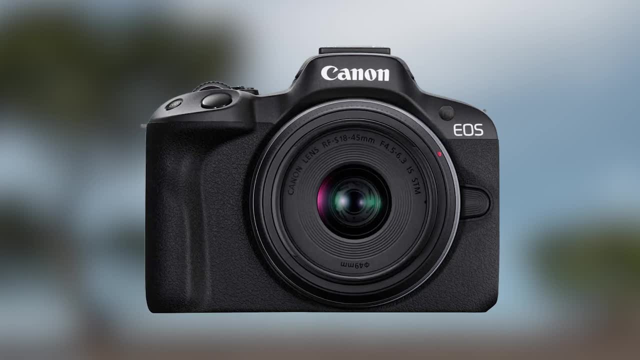 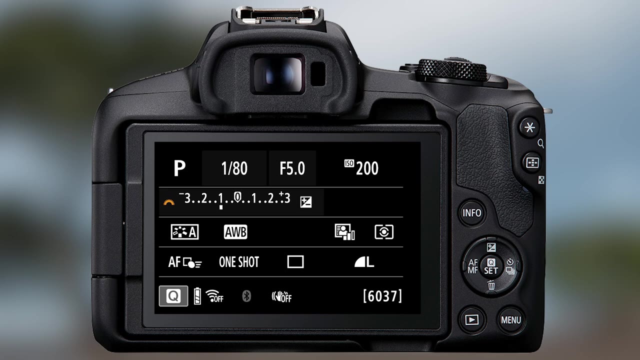 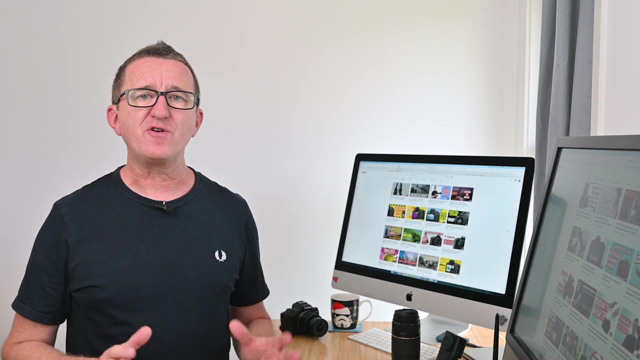 doubles the exposure and likewise, a decrease of minus one stop halves the exposure. On this canon R50, pressing the exposure compensation and then turning the dial on the camera will again allow you to either over or underexposure the picture. exposure image using exposure compensation. now i've made over 250 photography videos that you